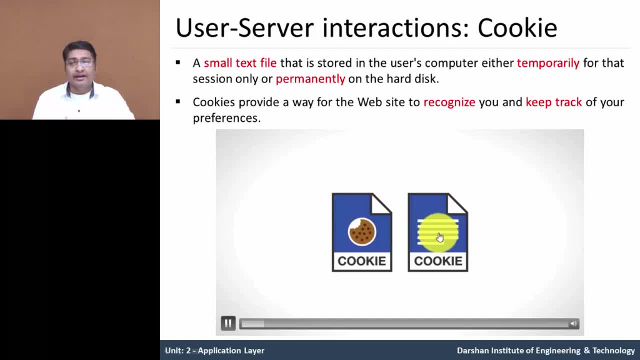 Which is stored in the user computer. Cookie is a small text file Which is stored in the user computer, Which is stored in the user computer, Which is stored in the user computer, Which is stored in your hard drive When you are visiting any of the website and choose the language preference as a English. 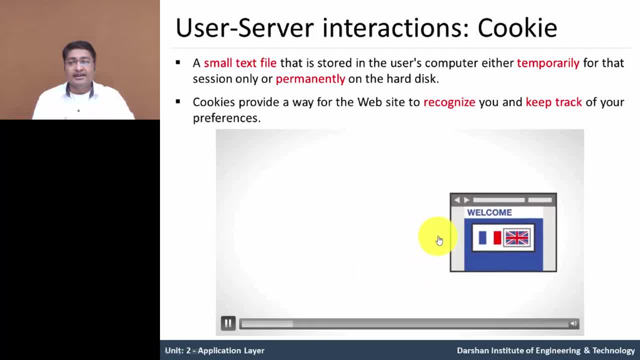 rather than other language. So that website set a cookie means stored cookie in your hard drive as a English language preference. After sometime again visit the same website, it set English website as English language preference website by default because cookie is already set as a English language now as 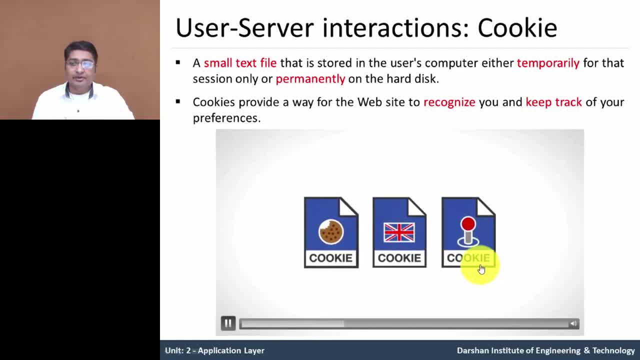 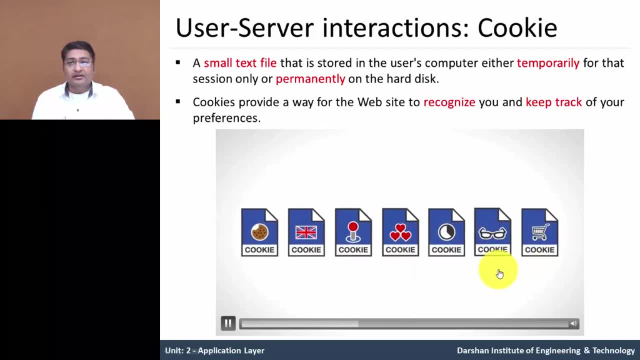 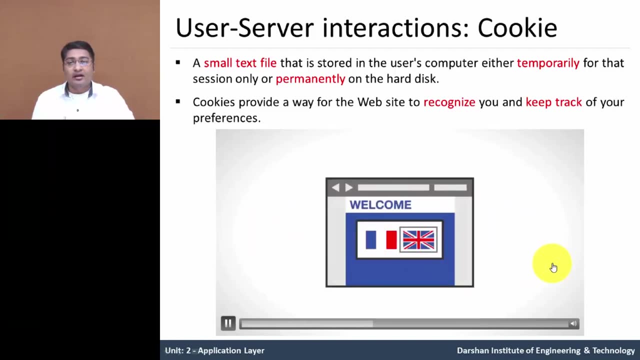 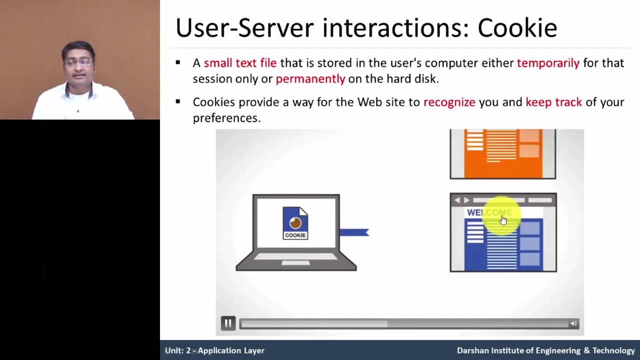 well as language, timestamp and like dislike, users activity, shopping preference and viewed link reference, stored in as a cookie. let's see another thing. if you visit same website, then your preference is set in English and the different website the first time you visit website, your reference will not. 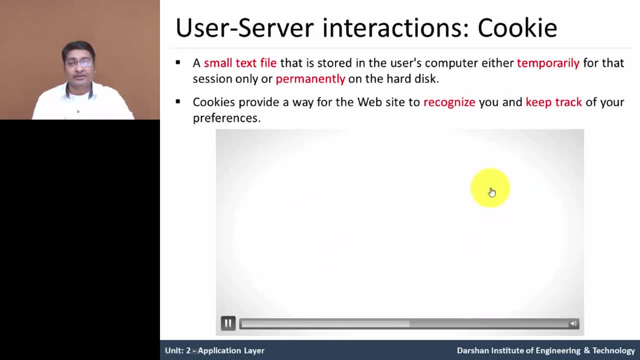 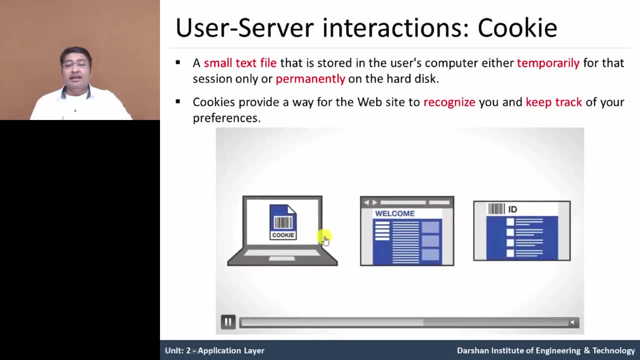 set as English because you're first time visited at that different website. now, after storing cookie, it said a ID number on server database. so, based on the id server, know the preference. let's see the example: when i will visit a visit a news website in news website. 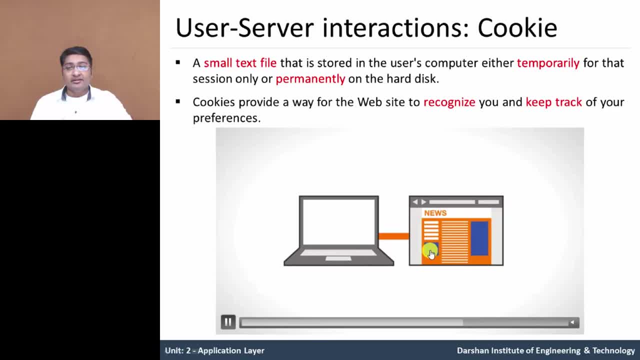 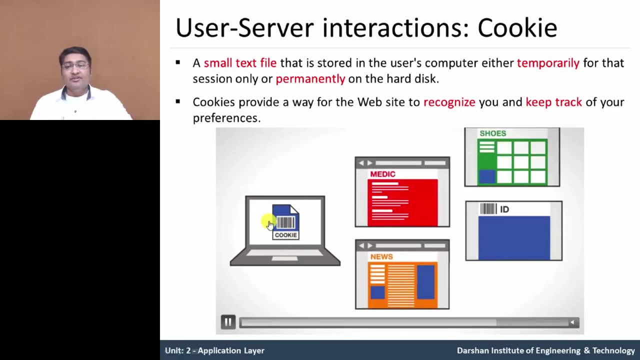 there is some portion for the advertisement of different site, so which content display over here? the content displayed over here is visited website by your computer. if you visit any of the shopping website or any health website or any entertainment website, so their content stored as a cookie in. 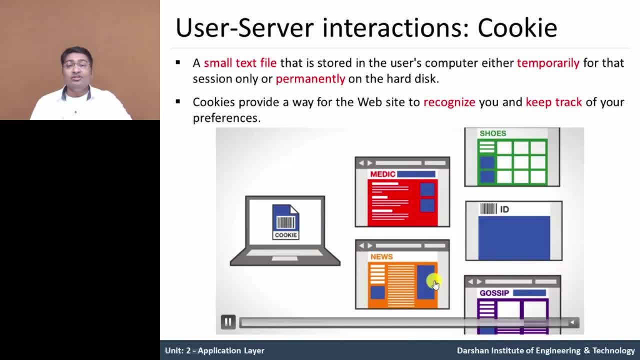 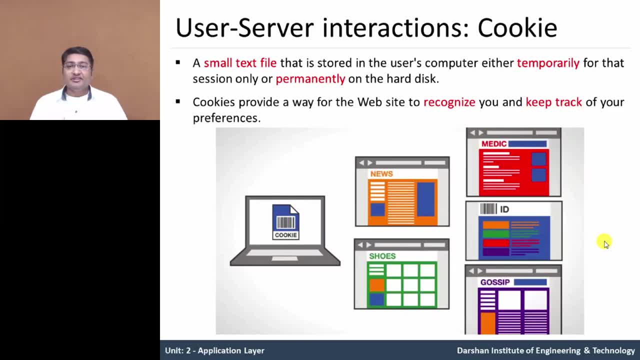 your drive, it will display on this particular site. let us see real example. you are facing same situation in day by day life. if you are visiting amazon website for buying shoes, after some time you are visiting any health regarding website. then onwards you visit news website. in news website, in this portion it display either amazon 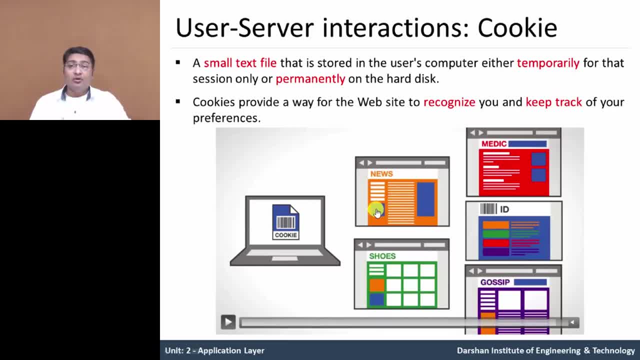 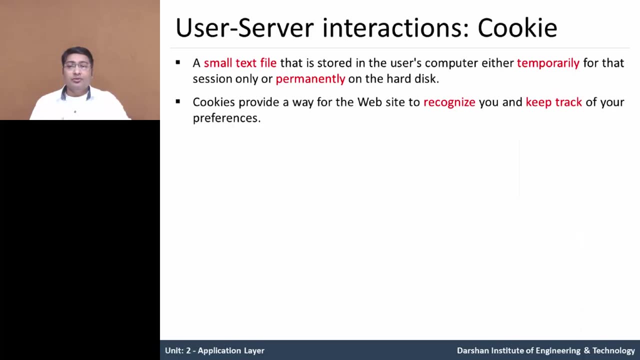 shoes content or medicine. regarding content or any of the visited website which you visit earlier. so it is come from the cookies which is stored in your computer. so cookie can contain four. part can say cookie has four component. first a cookie header line in http response message. so in http. 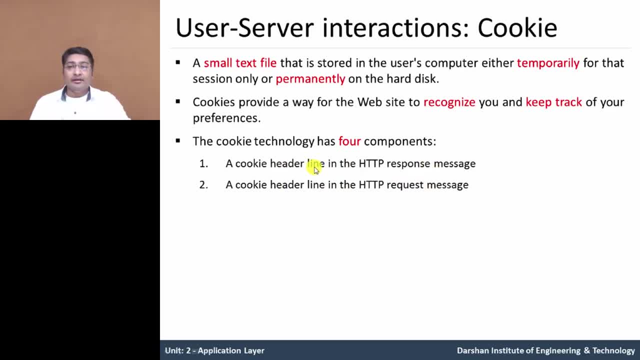 response message the cookie header line included as well as http request message. it also included a cookie header in http request message. third one is cookie file kept on the user end system and managed by the user browser. fourth one is a backend database at website server so it store a cookie id. 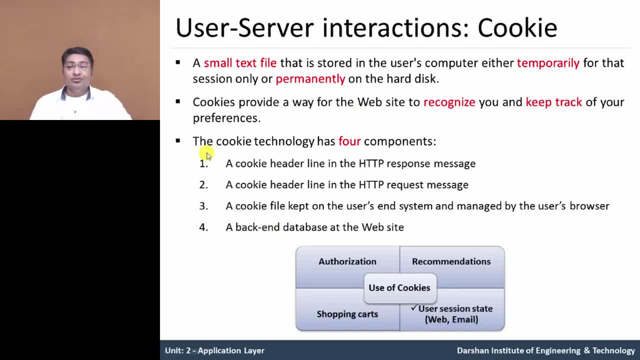 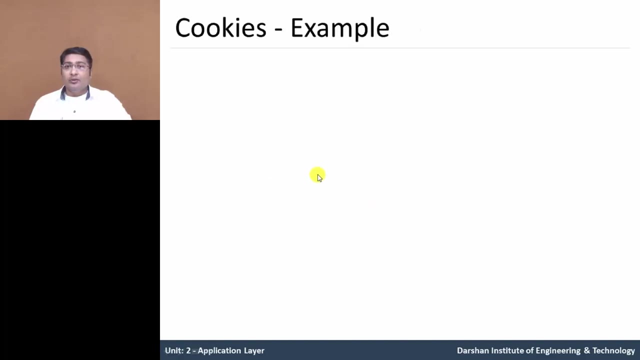 now what the use of the cookie. it is used for the authorization of the any users identification. recommendation means you set a preference of the any of the languages in particular. website shopping cart items, session details about email, email or any of the website. now let's take an example. 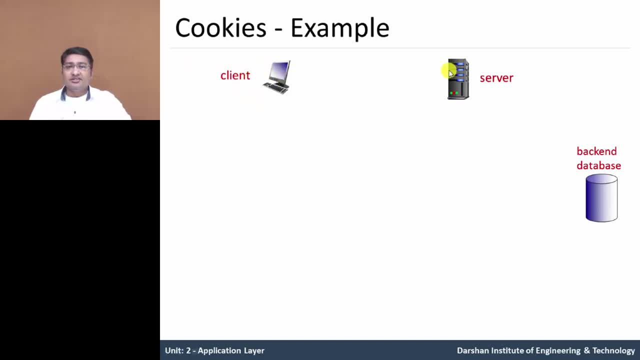 here in this figure the client server and backend database of web server. now client visited a website shopping website, ebay. so the ebay cookie stored in client computer and id of the ebay cookie is 8734. after time client visited first time second shopping website. it is a amazon. 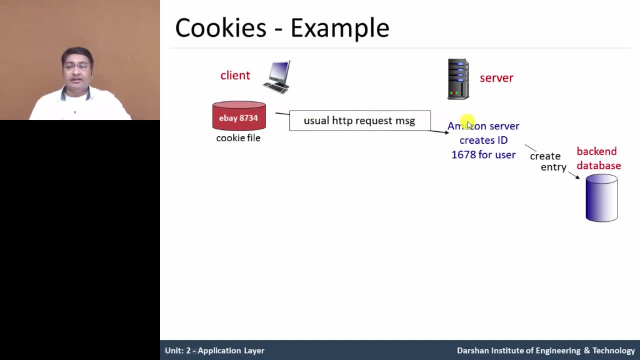 so first time it visited amazon website the client make a connection and then send http request message to the server. amazon server. it create a cookie id 1678 for the user and that cookie id entry stored in the database of server. now amazon server reply response. object: page with cookie id 1678 to the client side client. 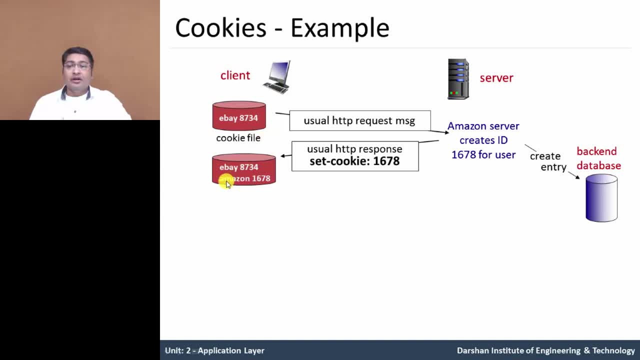 browser stored amazon website cookies id 1678. after some time or second time, client send again a request for the same amazon web page. see the http request message from the client for the cookie means same web page. you click on the same website and you have entered the same id, 1678. 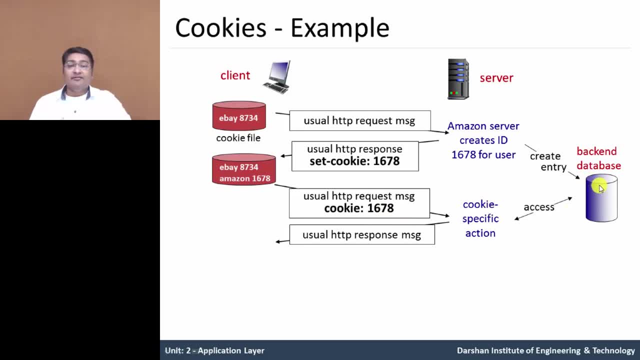 so the server receive reference id 1678 from the database and reply the response message to the client. after one week again I want to access same website, Amazon. so in this example it will create cookie again or not? no, it not create again cookie ID because it already stored. 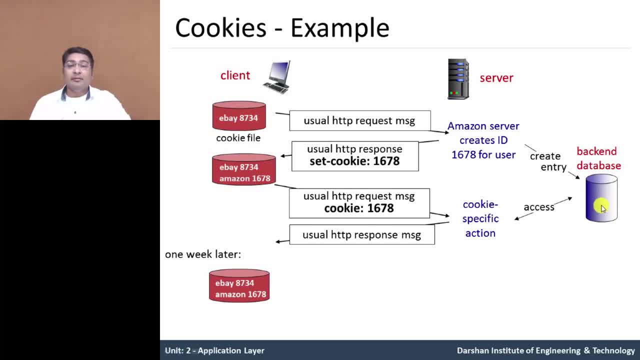 previously on this back-end database. let's see client send a HTTP request message with cookie ID 1, 6, 7, 8, which is stored earlier, and the server reply that cookie ID with response message to the client. 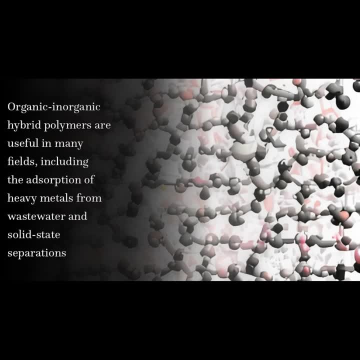 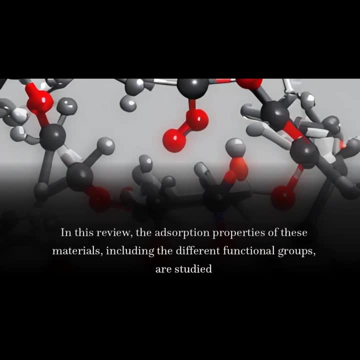 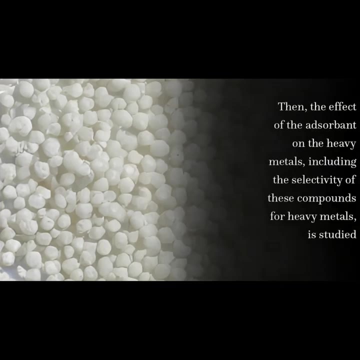 Organic-inorganic hybrid polymers are useful in many fields, including the adsorption of heavy metals from wastewater and solid-state separations. In this review, the adsorption properties of these materials, including the different functional groups, are studied, Then the effect of the adsorbent on the heavy metals, including the selectivity of these. 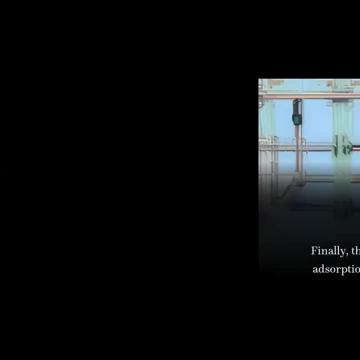 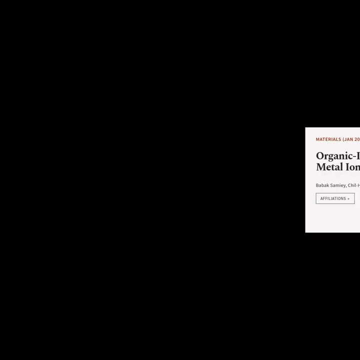 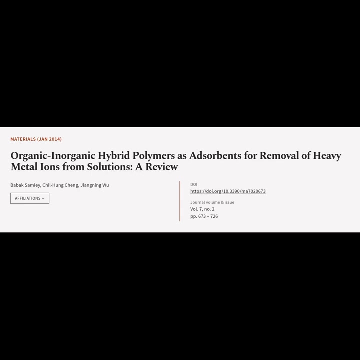 compounds for heavy metals is studied. Finally, the effect of pH and synthesis conditions on adsorption capacity of these materials is discussed. This article is titled Organic-inorganic hybrid polymers as adsorbents for removal of heavy metal ions from solutions, a review, and was authored by Babic Samyi.